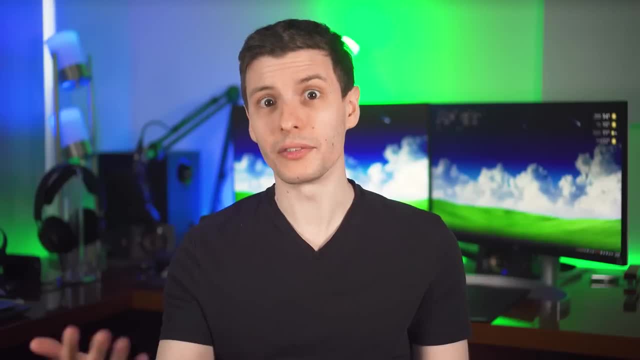 including by Googlecom. So if you want to know more about how to report malicious websites, you can go to Google Safe Browsing. So being vigilant is always the key, though it still is worth it, in my opinion, to add as much security as possible. 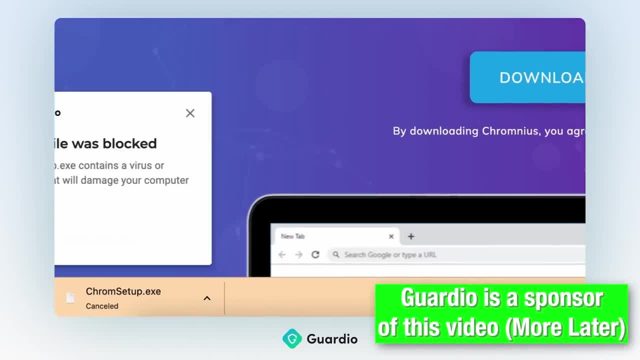 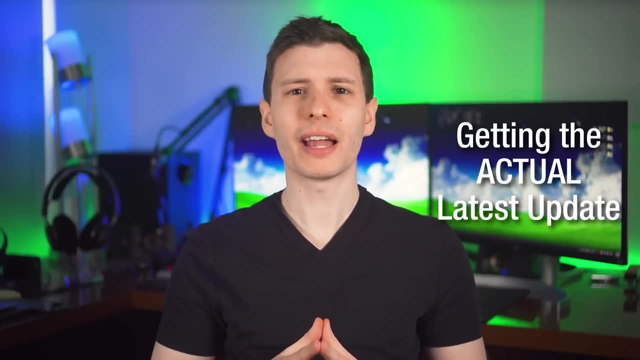 And actually a bit later I'll also talk about the video sponsor, Guardio, which is another great way to fill security gaps like that that aren't covered otherwise. Next up, this is one that probably not a lot of people realize, and that's, if you're. 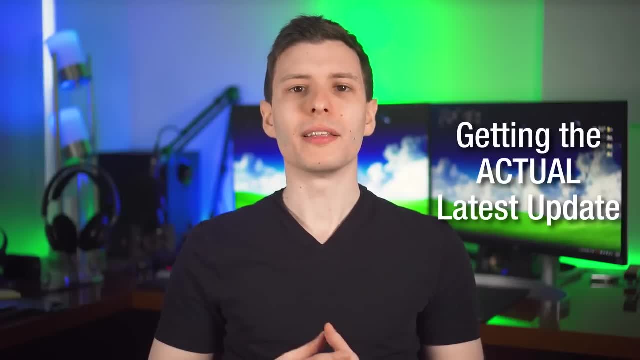 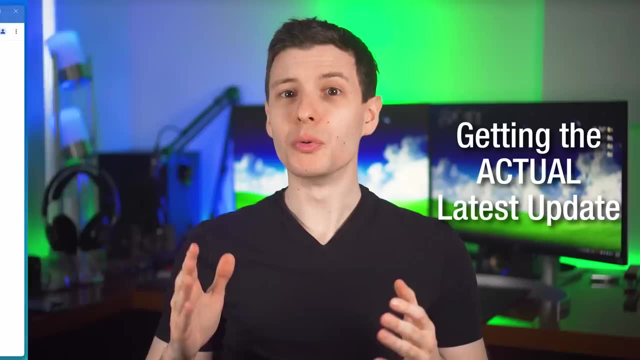 using Google Chrome and you want the latest update, like a patch for a zero-day exploit. Yes, you can just wait for the browser to auto-update, but you probably won't get that patch as soon as you can, as if you were to go and manually check for an update. The only way to 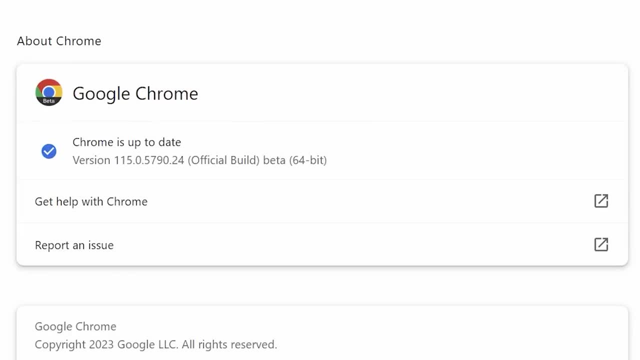 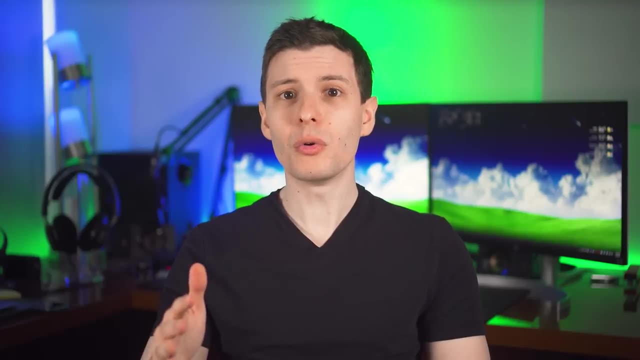 guarantee that you're actually on the latest version of Chrome is to do a manual update, because Google does staged rollouts of auto-updates to users. Even though Google Chrome does check automatically in the background for updates, they put people in different cohorts. 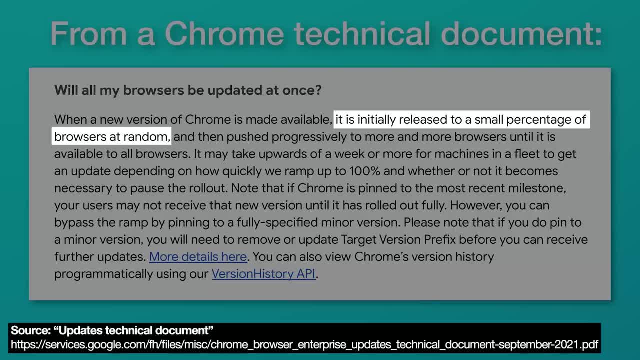 they're called, which are basically groups that you're kind of randomly assigned, where after they release a patch onto their servers, a small group of people will get it immediately On auto-update, but some people- a large group- may get it days or even weeks later. 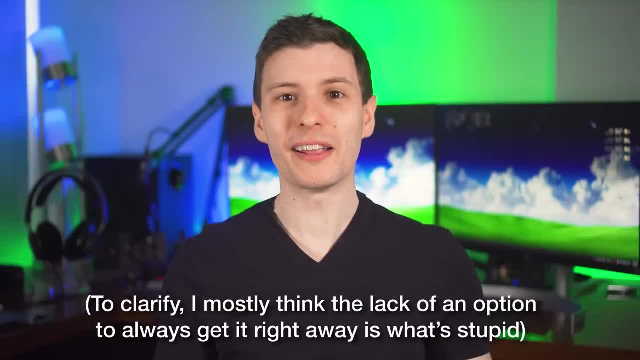 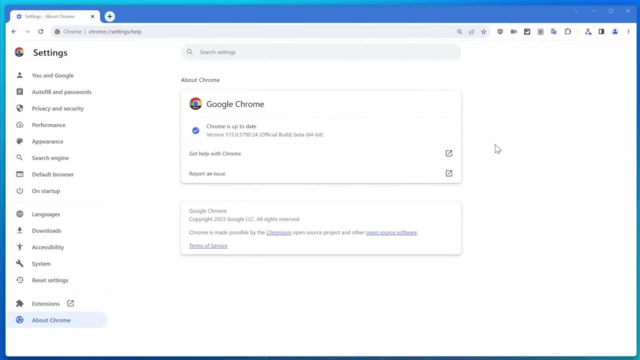 which is stupid in my opinion, And there is no setting or anything to tell Chrome. no, I always want the latest update right away. So you literally have to go to the about page or the version info page of Google Chrome and then it will always manually check for the latest. 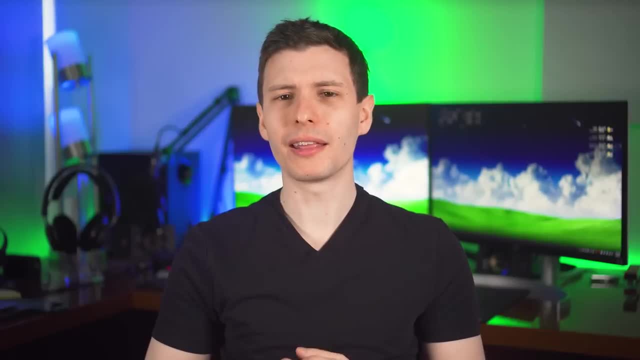 update and bypass that staged rollout thing. From my understanding, this is a Google Chrome specific thing. I do not believe, from what I've been told, that Firefox does this. it gives everyone the latest update right away, And I believe Edge and others probably do the same. 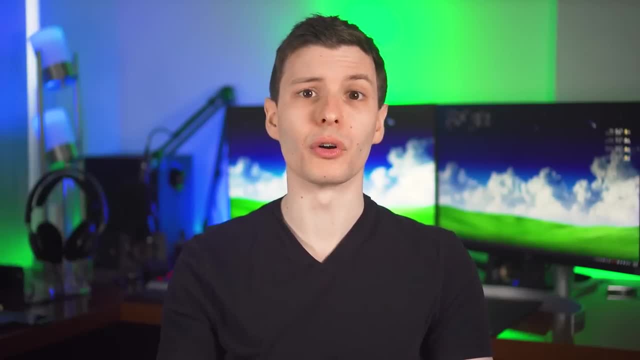 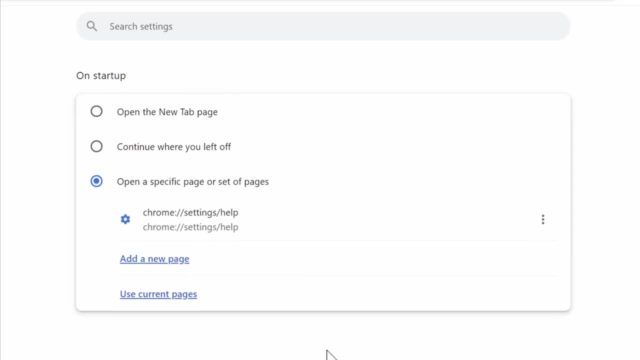 Now one thing you could do on Google Chrome if you don't really care about the startup page, is to set the startup site to the about page in Google Chrome And that way, every time you start up the browser, it'll auto-check for an update. 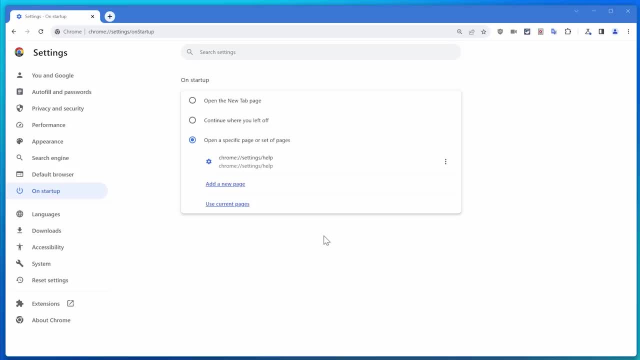 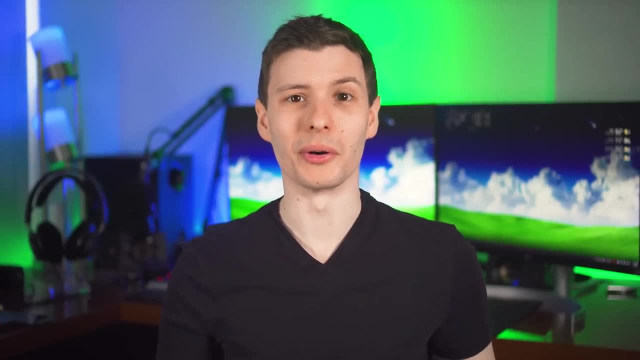 So you can do that in the settings under on startup, and then it says on a specific page and you can just set that to Chrome colon slash, slash settings, slash help. Otherwise you may be at the mercy of whenever the auto-update decides to get you the new version. 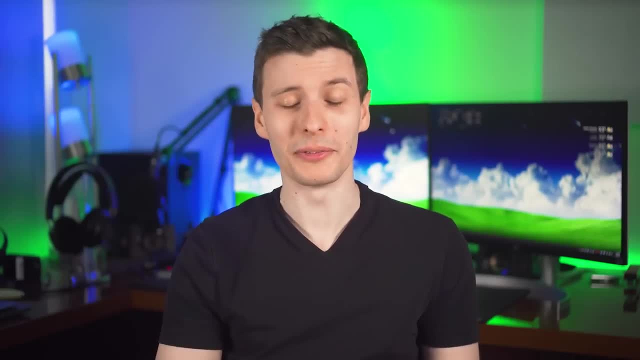 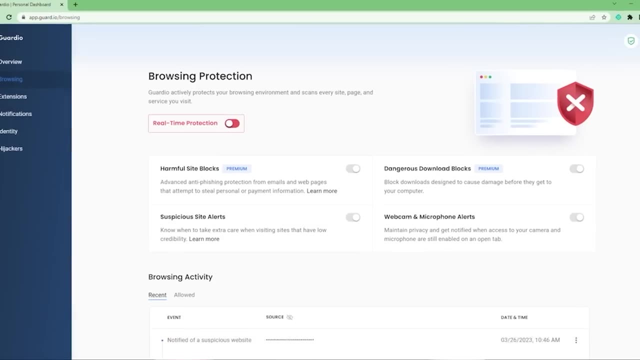 Now, on the topic of Chrome security, we have a very relevant sponsor for today: Guardio. Guardio is a browser extension that provides real-time protection from all sorts of threats while browsing the web. For example, it blocks malicious sites using in-house custom. 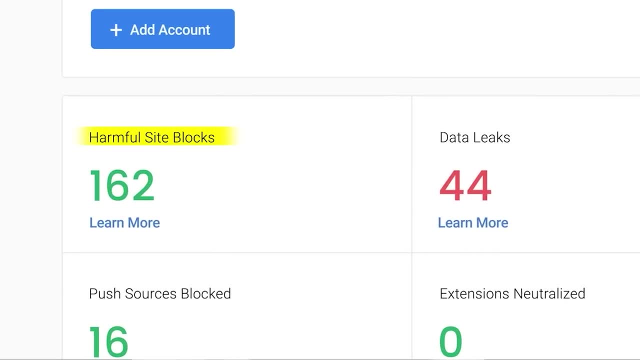 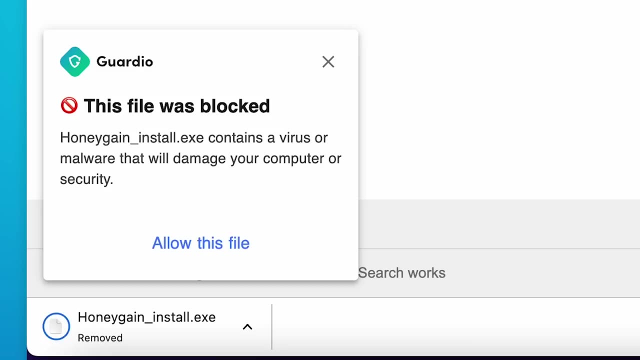 developed methods for detecting phishing and malware content all before those threats even have a chance to do any harm. Guardio has also added download protection to block malicious files, even if you accidentally click to download them, like from fake sites for popular software or even malicious sites for malware. Guardio has also added download protection to block malicious. 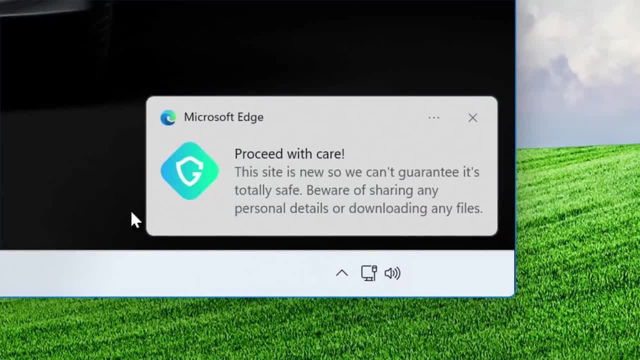 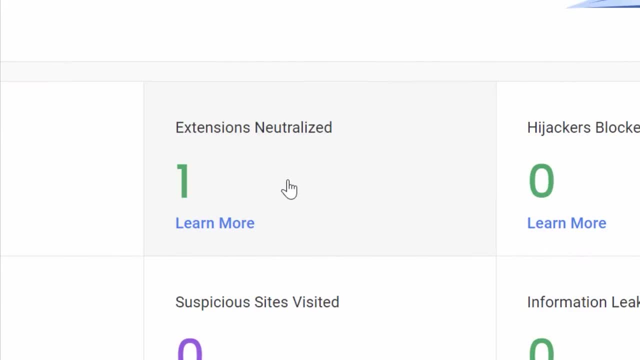 game mods. One of my personal favorite features is that it will warn you if a website's domain has been registered very recently, which is a major red flag. Guardio also scans your other browser extensions and alerts you if there are any disguised malicious extensions installed. 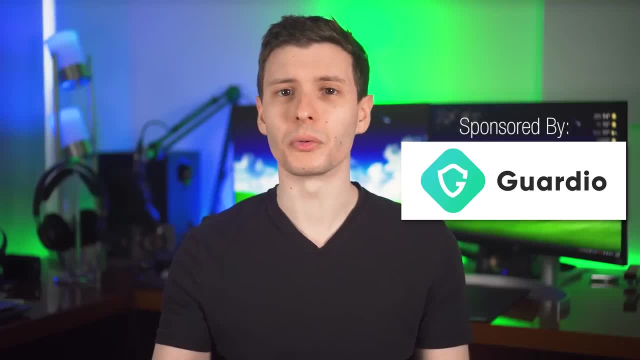 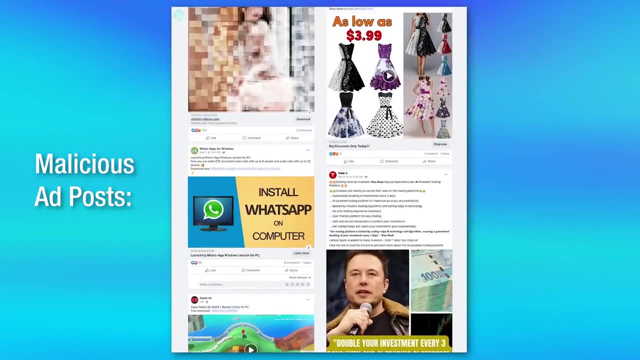 and disables them, And they really know what they're doing. They even do original research on new attack vectors and recently published an article about hackers using paid ads on Facebook and Twitter to spread malware, a technique they call malware posting, which Guardio can protect. 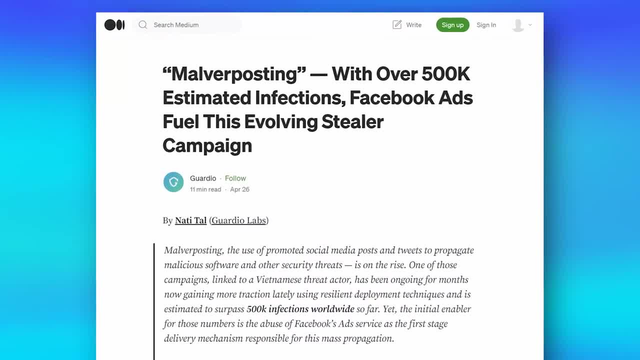 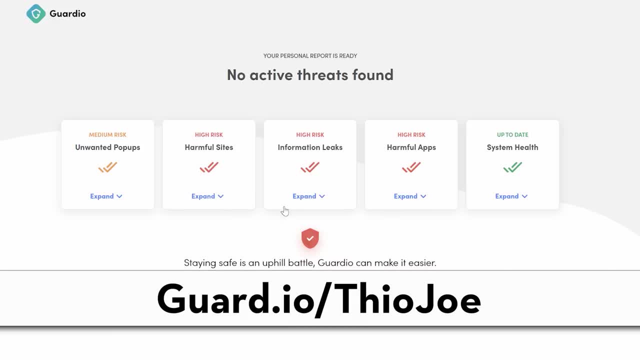 against, of course, And I'll put a link to that article in the description if you want to check it out. You can scan your browser for threats for free by visiting guardio slash theojo and installing the extension, and you'll also get a free 7-day trial to their premium features, such as real-time. 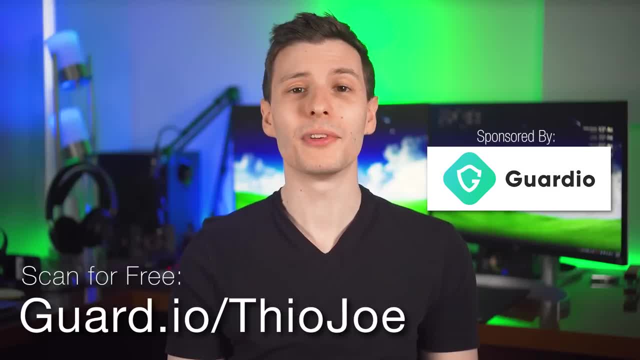 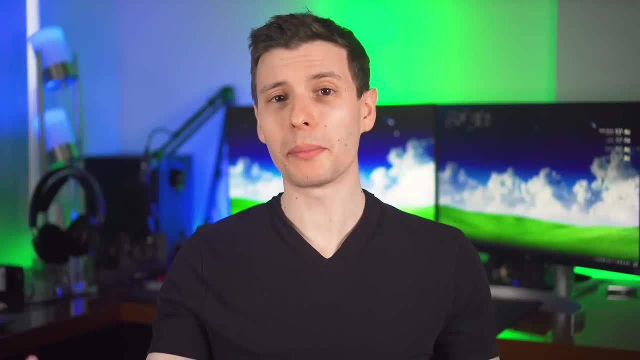 threat removal. So if you want a clean and secure browsing experience again, visit guardio slash theojo link in the description and also check out their affordable premium plan for full protection. And with all that being said, let's continue. All right. next up, we have a setting. 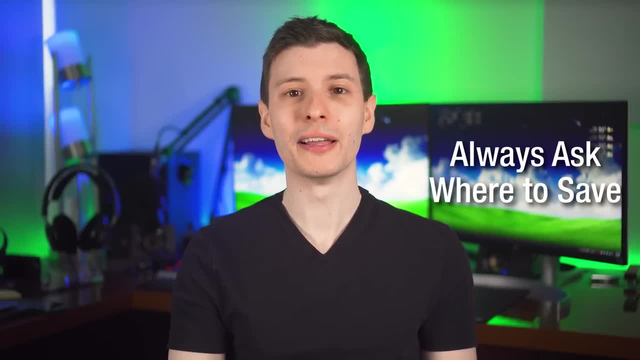 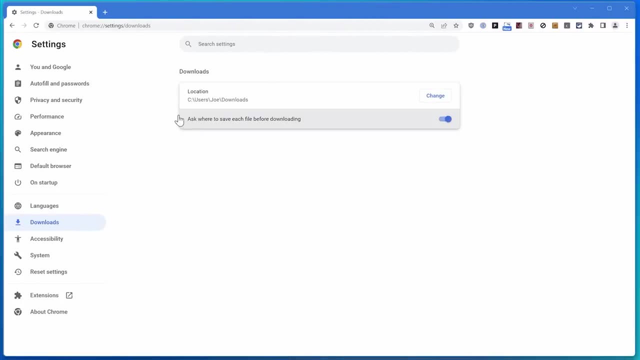 that is personally one of the first things I change on any web browser I install, and that is to always have the browser ask to where I want to save a download. You can usually search your browser settings for downloads and it'll be somewhere in there And in Chrome. 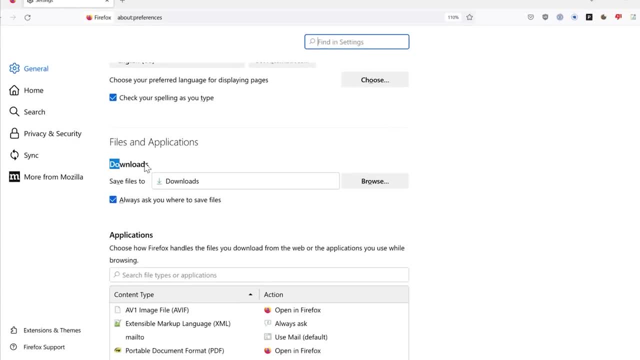 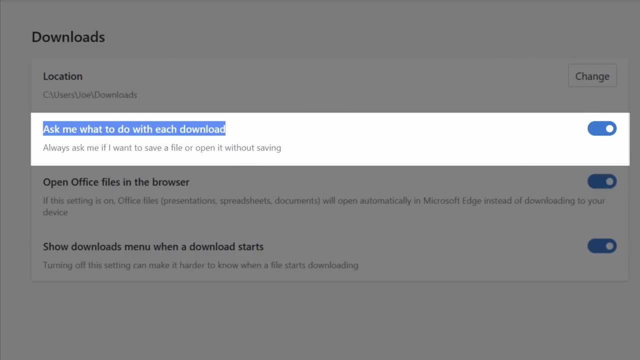 for example, it's called ask where to save each file before downloading, and on Firefox it's called always ask where to save files, And Edge has a similar setting. The benefits of this should be pretty obvious, but sometimes you don't necessarily want to just download everything into. 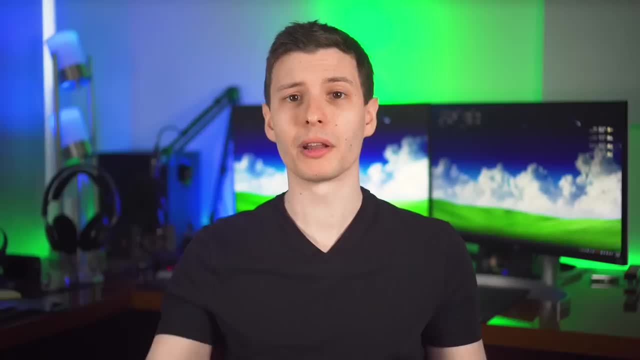 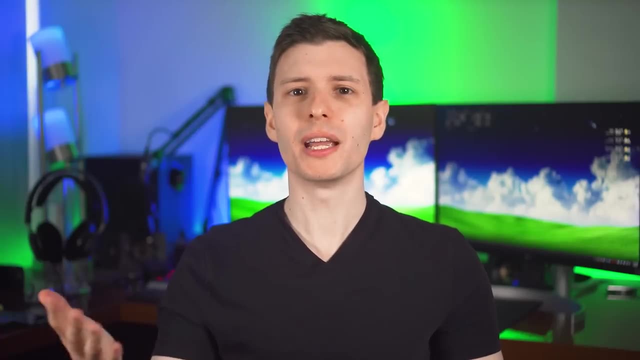 the downloads folder. Like if you're downloading a document, maybe you want it to go right in the browser, but if you're downloading something from some browsers like Microsoft Edge, if the webpage initiates a download, even if you didn't necessarily want a download, the browser will just. 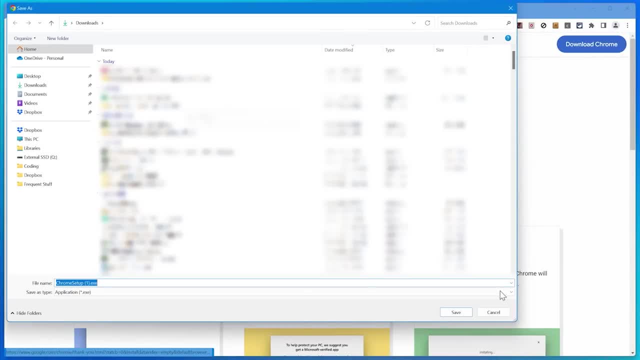 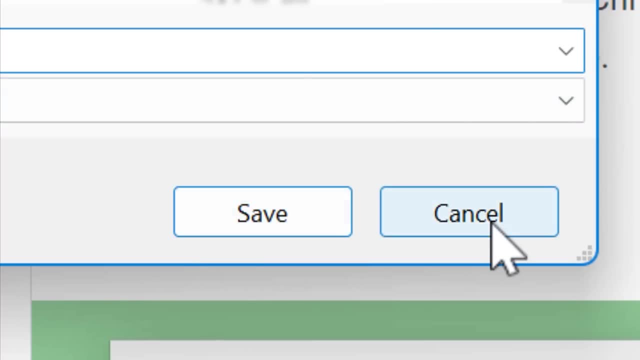 automatically start it. So this way it'll just pop up an Explorer window and ask you where to put it, and it'll probably just default to the downloads folder anyway. So you can just click save. It's not any more difficult. And then, if you want to put it somewhere else, that's how you do it. 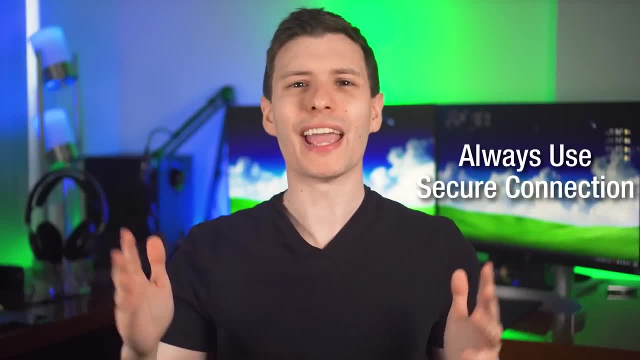 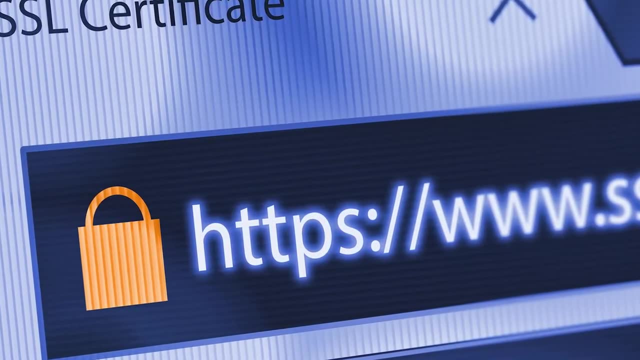 You can always use a secure connection For context. basically every website these days should support encrypted connection or HTTPS, And it's really the exception. if they don't, that's a very outdated website, But there are some websites that they may support HTTPS. 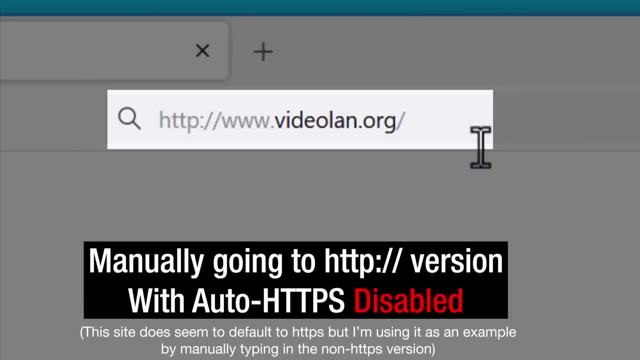 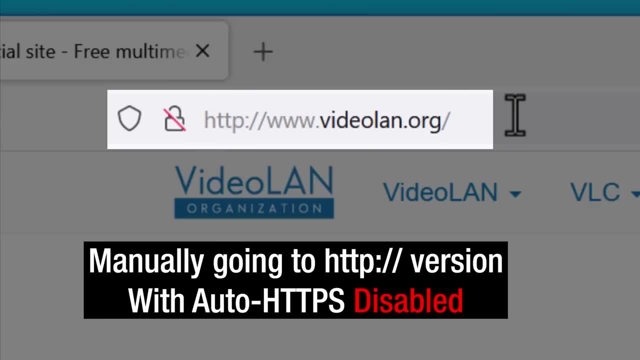 but if a user goes to the website, it was default to not encrypted and you probably want to use the encrypted version if it's there. So that's basically what the browser will do with the setting: If it detects you're going to an unencrypted. 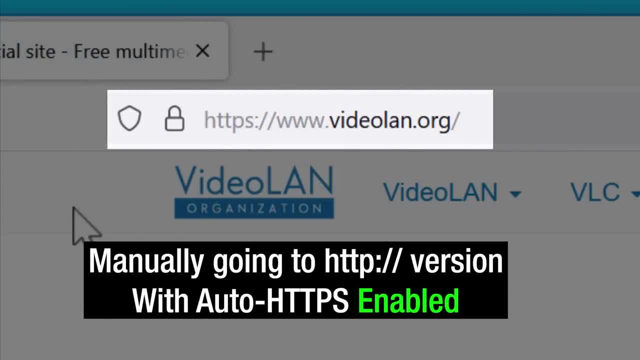 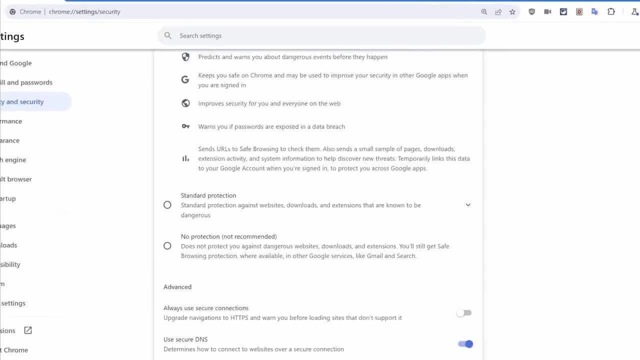 website, it'll check if there is an encrypted version and automatically go to it. I do know that if you visit a website that doesn't support encryption at all, then it will obviously show warning. On Chrome, this setting is called always use secure connections, and you can just search. 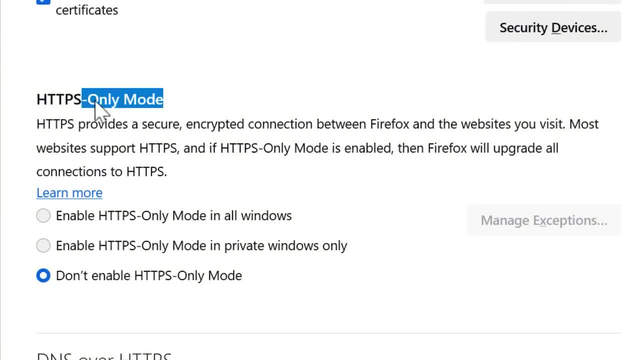 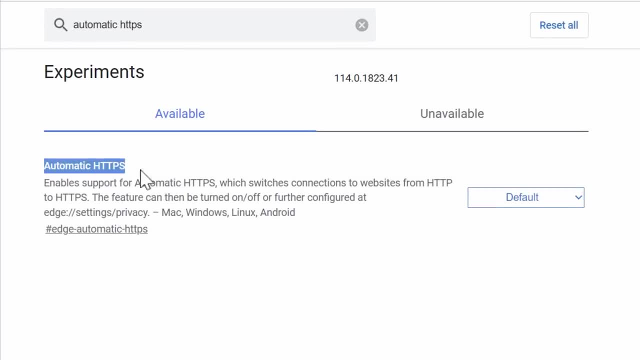 for it On Firefox. it's called HTTPS only mode and I would just set it to always. use it. Now for Edge to even enable the option, you have to go into the Edge flags menu and do a search for automatic HTTPS and enable that. 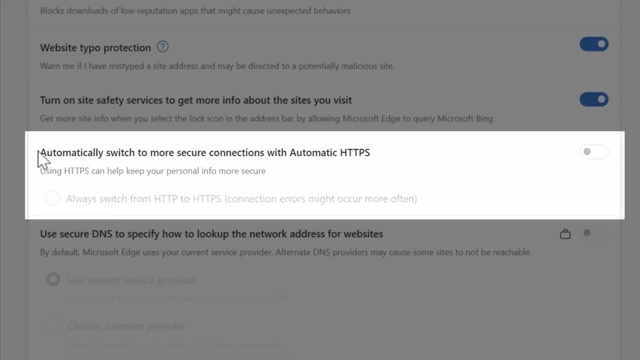 And now the setting will show under security and it'll appear as automatically switch to more secure connections with automatic HTTPS. Now, strangely, it seems like you can't toggle it on, but if you click on the text here specifically, it then turns on. I'm not sure what that's about. 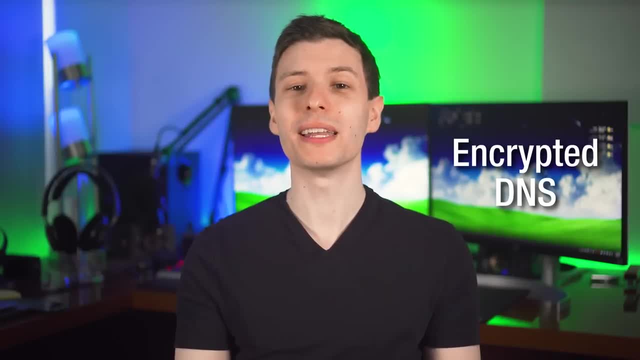 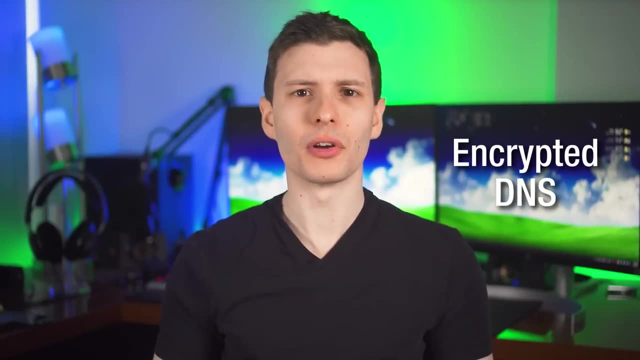 but that's how to do it. Now, speaking of encryption, next up, we have encrypted DNS, and pretty much every web browser these days has an option for that, but it might not be on by default. If you're not familiar, a DNS service is basically what the browser will use when you type. 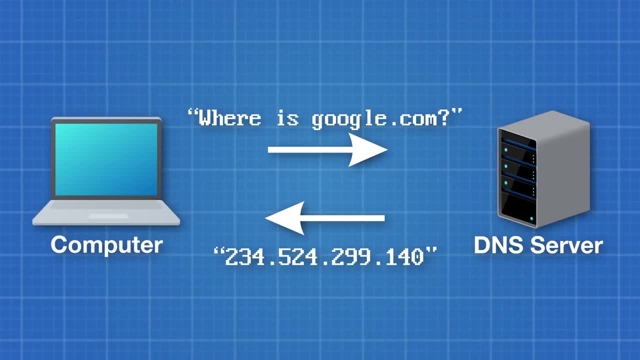 in a website name and then you type in the name of the browser and then you type in the name of the browser. and then you type in the name of the browser and then you type in the name of the website. It will use that to convert it to the IP address of the website that the browser can. 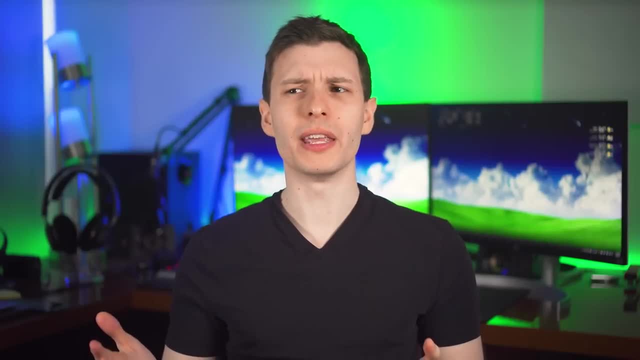 actually use for the connection, But for the longest time, even if the connection to the website was encrypted so no one could see what you were doing. the connection to the DNS service was not, which means that a ISP or whoever could snoop in and see what websites you're. 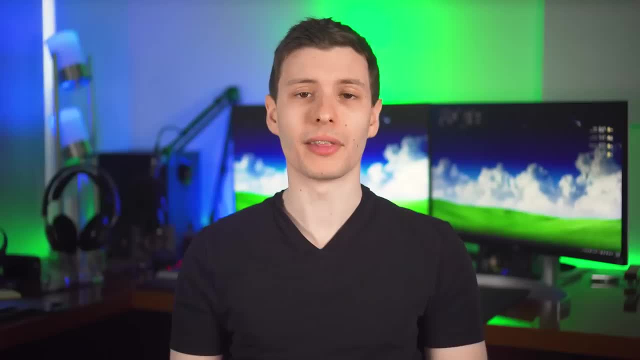 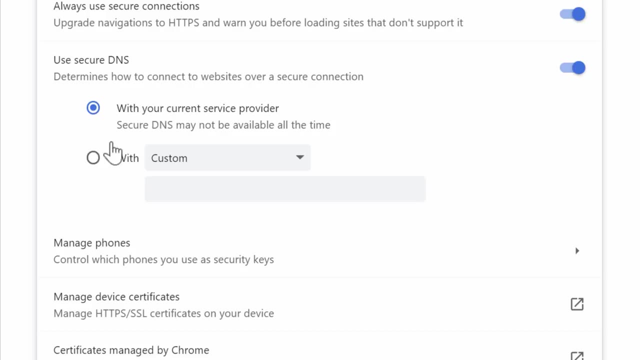 trying to connect to With encrypted DNS. this help protects against that, though. In Chrome you can get to this by going to settings and then privacy and security and use secure DNS and just make sure that's enabled, But be aware that by default, I believe this will. 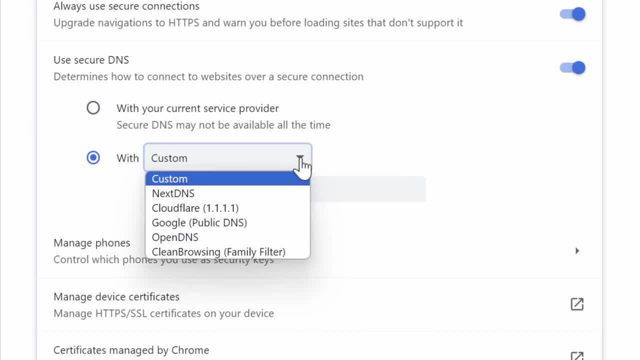 still use your internet service providers DNS servers which may not even support encrypted DNS, So you should probably use a third party DNS service that usually are better. Chrome actually has some options built in right there that you can choose from. I would recommend either Cloudflare or NextDNS, Though, if you're someone who already configured, 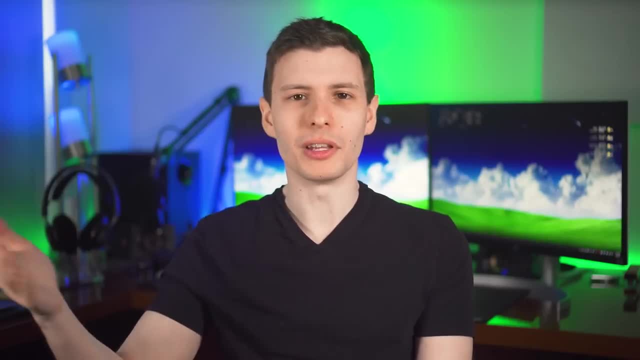 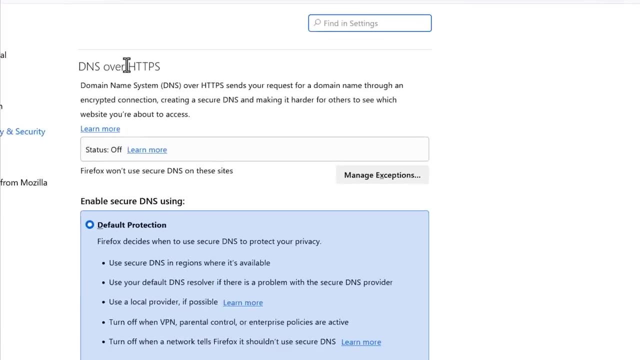 third party DNS at the router level, for example. obviously you don't want to do that here because that would override that, But you probably already know that if you're that person On Firefox, you can find the same setting by searching for DNS over HTTPS. it's the same thing. 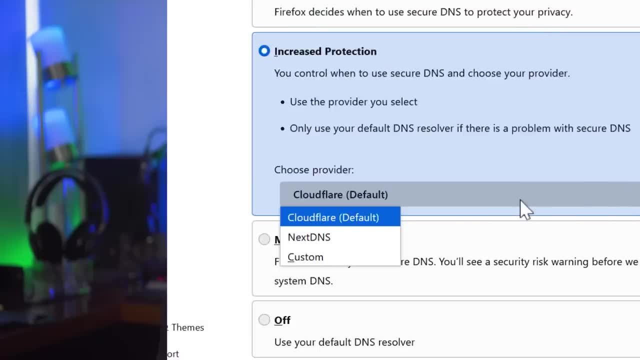 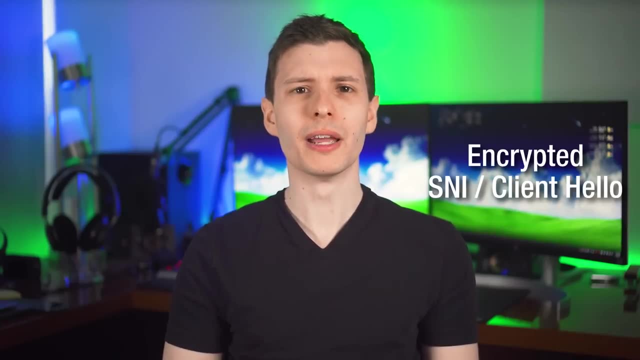 And just choose either increased or max protection, And again it gives you a couple options you can choose from. Now, speaking of encryption, again here's another setting that probably very few have heard of, and that is encrypted SNI. This might have a few related names. One is SNI, which stands 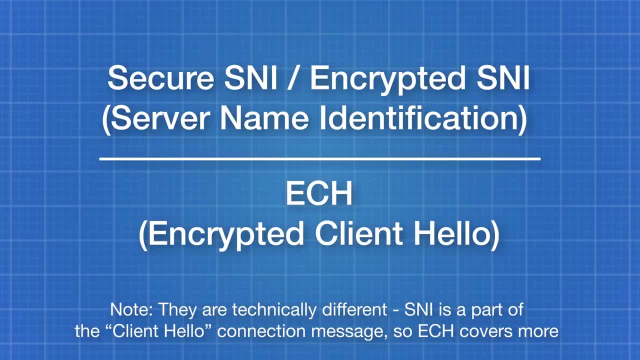 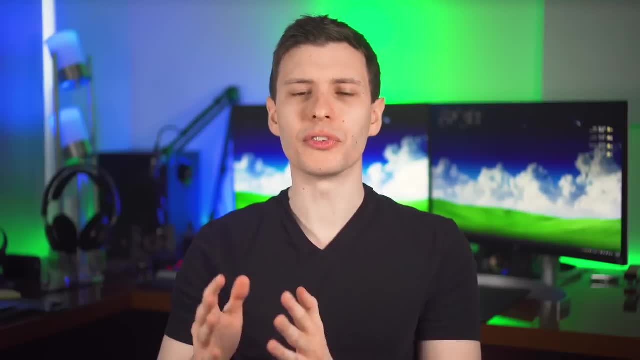 for server name identification, The other one- it might be called something like ECH- which is encrypted client hello, And basically what this does is prevents anyone from snooping in and being able to see what website you're making an encrypted connection to, Even though 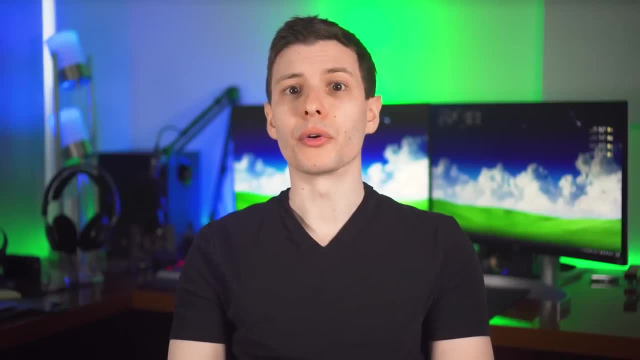 they can't see what's going on inside it. they can at least see what you're connecting to, And this is slightly different from DNS, because DNS is basically looking at the IP address, whereas this is like just connecting directly to the website, but the privacy concern is the same. 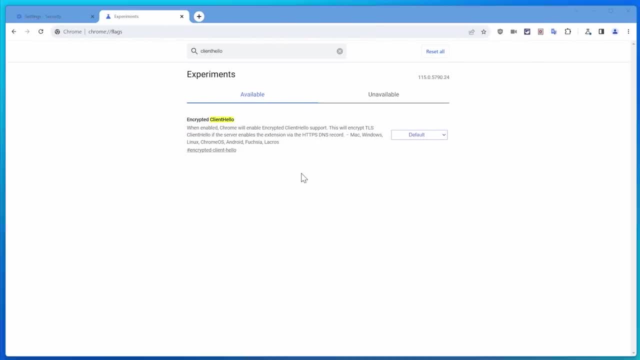 Now, to enable this, you need to go into some advanced settings. So if you want to enable this, you need to go into some advanced settings. So in Google Chrome you're going to need to go into the Chrome flags menu and then search for encrypted client hello and then enable that. 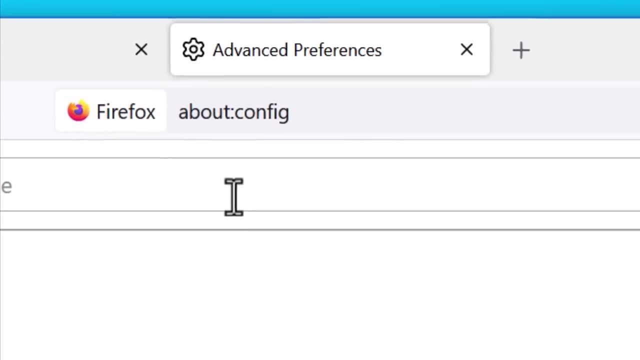 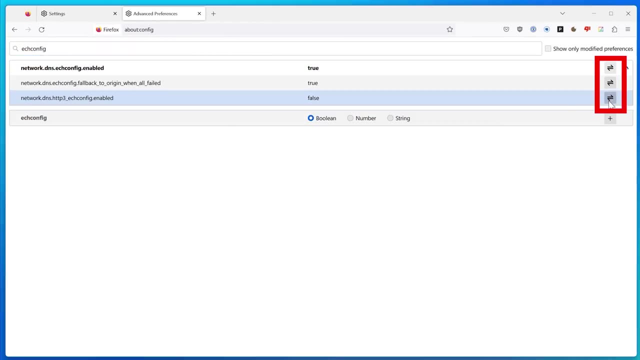 And in Firefox you need to go to the about colon config menu and then click show all and search ECH config and then toggle the following to true by clicking the thing on the right You want to do: networkdnsechconfigenabled, and then the other one. 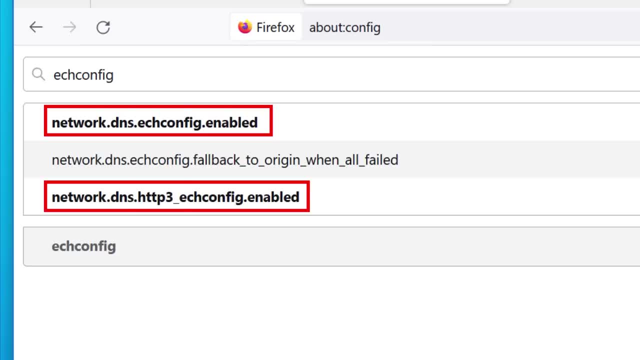 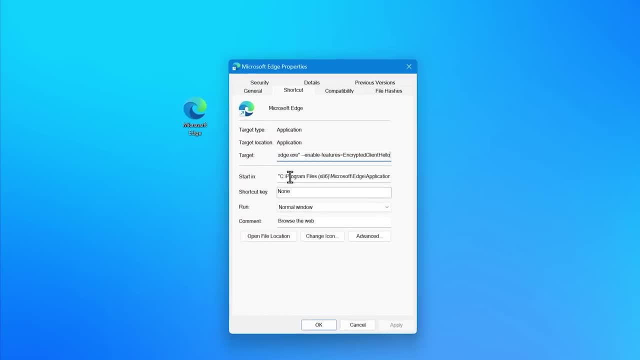 networkdnshttp3.echoconfigenabled. Now for Edge. technically it does support this encrypted client hello thing, but it's a bit complicated to enable. First you have to change your desktop shortcut to add the following parameter: to enable the feature. And if you don't use that shortcut, it won't be enabled. I don't know why there's no way to toggle it permanently. Then you'll also need to go into the flags and search for use DNS, HTTPS, ALPN and enable that as well, And now it'll work. Though, for all that work it's probably not worth it, especially 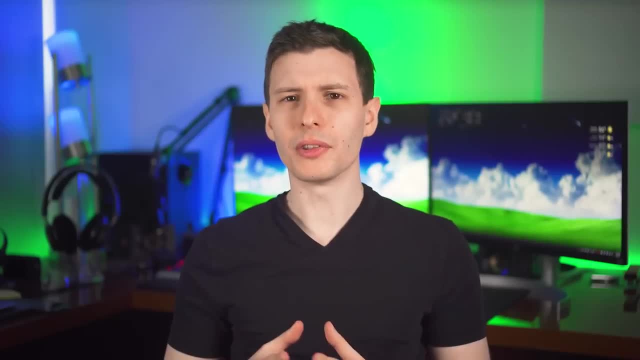 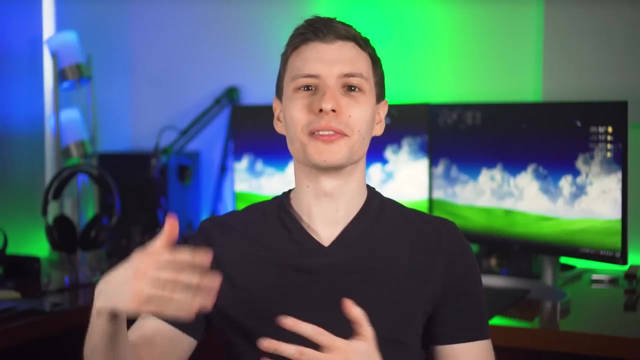 considering it's not really used much yet. The reason I believe this is not enabled by default is because the specification is not finalized yet and not a lot of websites really support it. There's very few. but I don't see a reason not to enable it, because at least you'll know if it does. 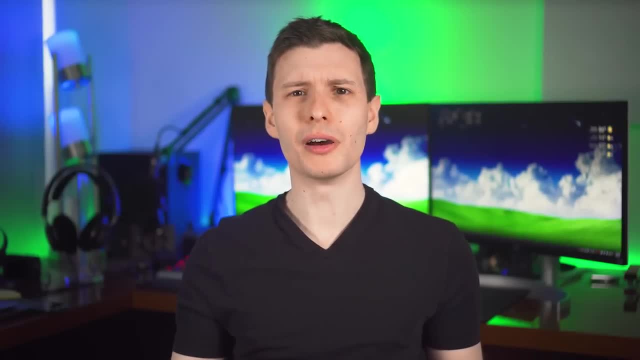 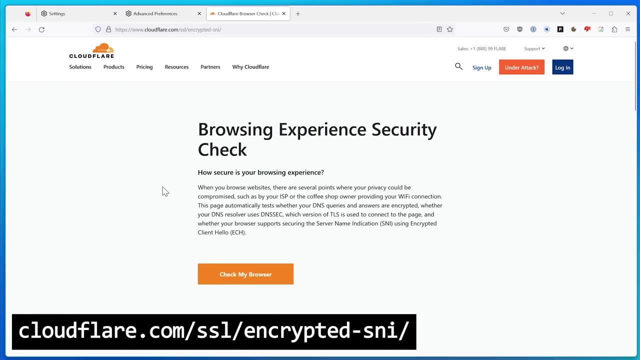 ever finalize, you won't have to remember to enable it. It'll be good to go. And if a website does support it, you can still use it. And you can test to see if this is working by going to a test page by Cloudflare. I'll put it in the description, but basically you can see on the 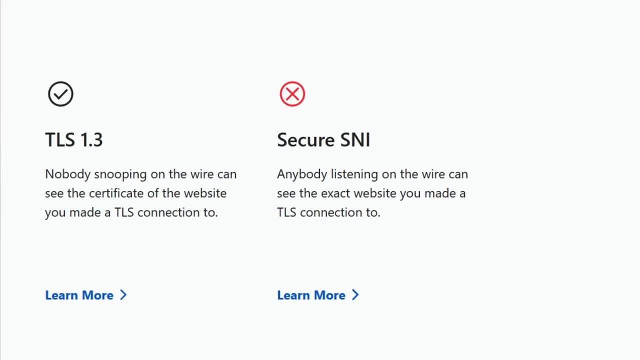 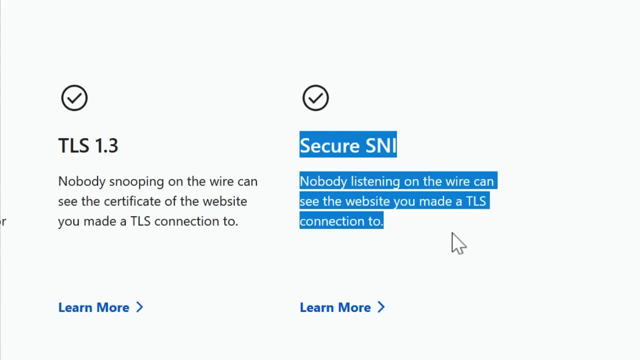 right if it says secure SNI and by default it'll probably say that it's not. But if you have the site enabled and you're also using a DNS service like Cloudflare or NextDNS that support it, it should show up as a check and working. after that, Though I will note, for some reason. 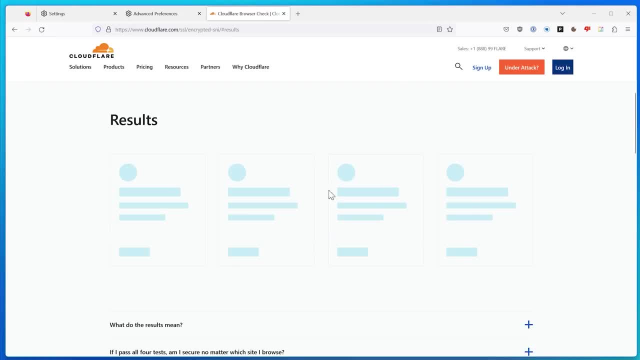 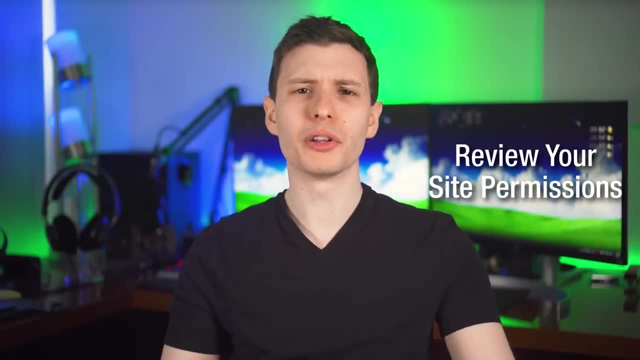 when I had my DNS set to Cloudflare, for whatever reason, the page test wasn't loading, but it did when I used NextDNS, So I don't know why that is, but you may notice that. Finally, this is one you should probably do every once in a while, no matter what browser you have. 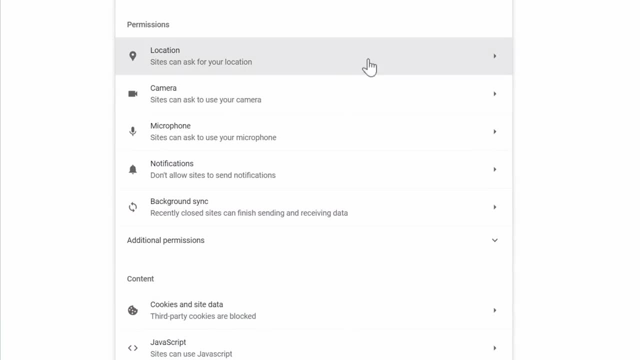 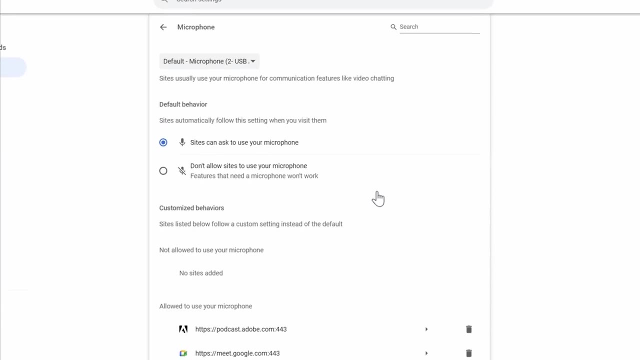 and that's review what site permissions you have granted. Chrome has a privacy section for this, and then in Firefox, privacy and security and then permissions. But basically just look through here and look at the various permissions and maybe see what websites have been granted that. 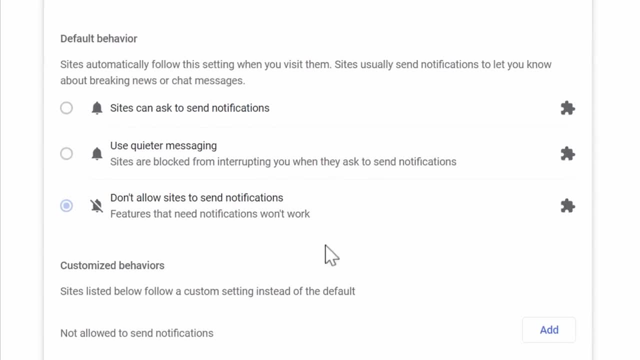 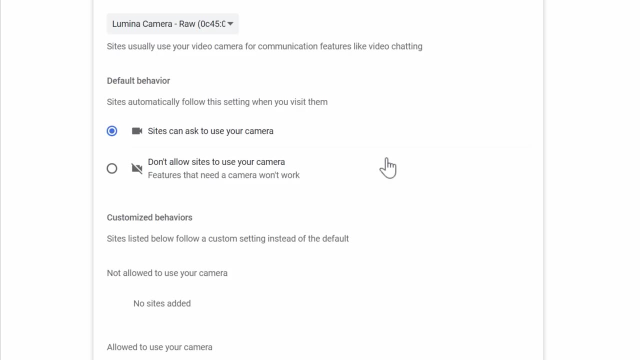 or you can choose to just not even allow websites to ask. For example, I don't use notifications on Chrome, so I just don't even allow websites to even ask about. But you might also want to look at, like the microphone and camera permissions and make 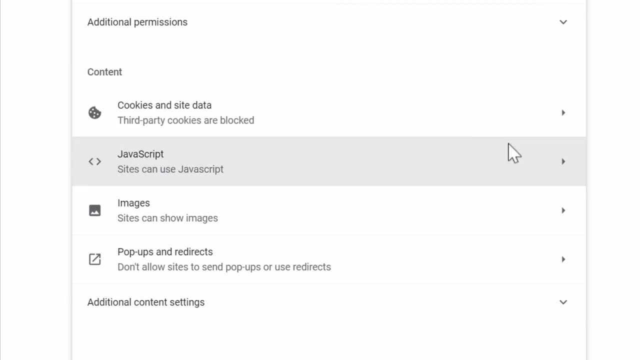 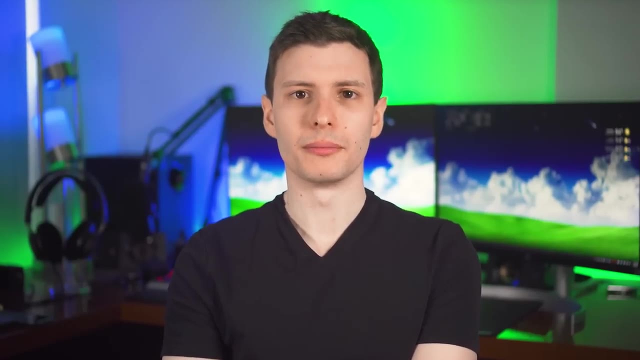 sure that there's no websites on there that maybe you accidentally enabled at some point and you don't want them being able to see your camera or microphone, And then you can do that for the other permissions as well. So at this point your browser should be a bit more secure than it was before.